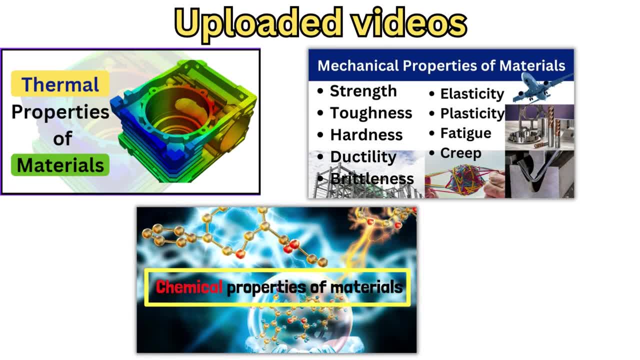 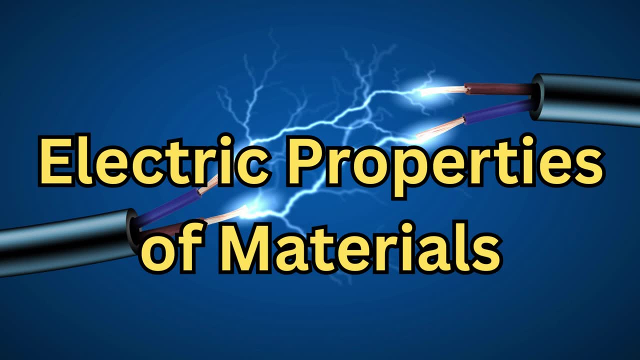 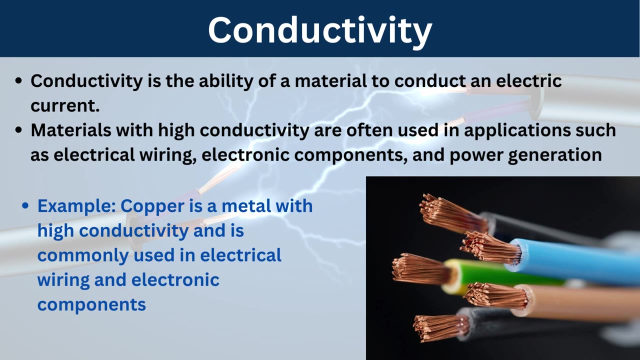 Hello friend. already we have uploaded the videos on mechanical properties of material, thermal properties of material and the chemical properties of the material. In this video we will discuss the electric properties of the material. So let's start the video. The first electric property of the material is the conductivity. So the conductivity is the ability of material to conduct an electric current. 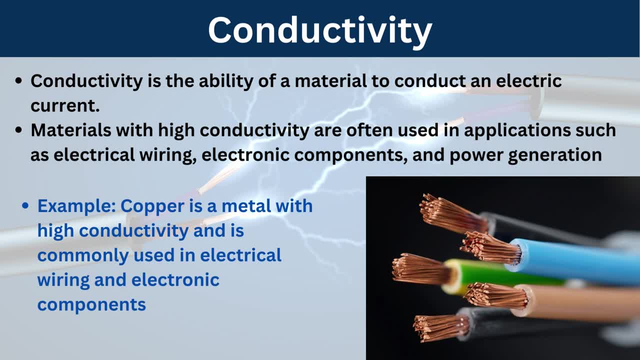 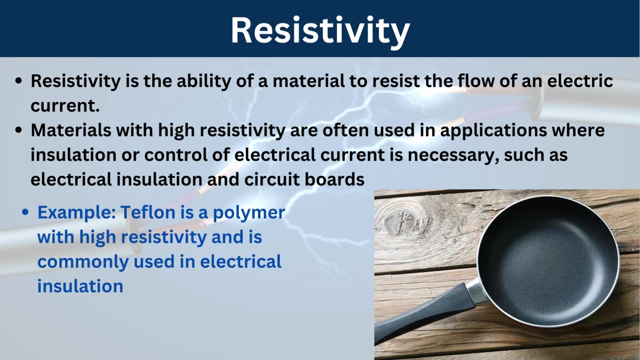 So the materials with high conductivity are used in applications such as electrical wires, electronic components and power generation. So you can take the example of copper. Copper is the metal with high conductivity and commonly used in electrical wiring and electronic components. Next electric property is the resistivity. 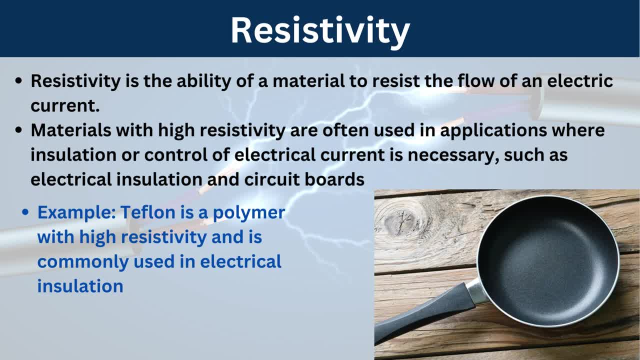 So the resistivity is the ability of material to resist the flow of electric current. So the materials with a high resistivity are used in applications where insulation or control of electric current is necessary, Such as electric insulation and the circuit boards. So you can take the example of teflon. Teflon is a polymer with a high resistivity and it is commonly used in the electrical wiring. 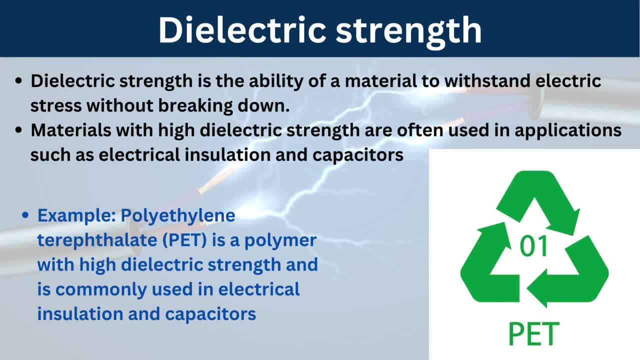 electrical insulation. next electric property is the dielectric strength. okay, so the dielectric strength is the ability of material to withstand the electric stress without breaking down. okay, so the material with the high dielectric strength are often used in the application, such as electrical insulation and the capacitor. okay, so you can take the example here: the polyethylene. 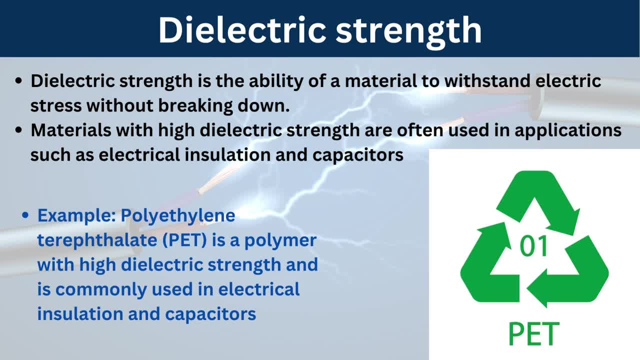 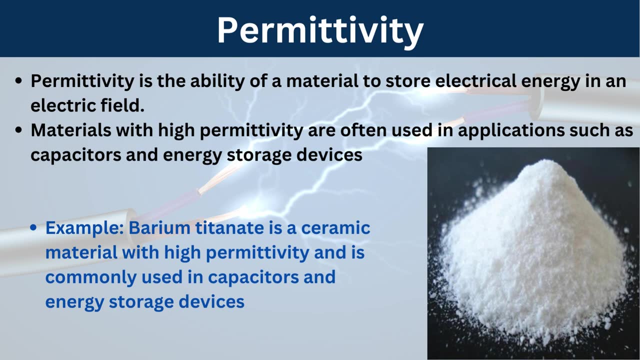 territorial- generally we call it as a pet- is a polymer with a high dielectric strength and are commonly use in the electrical insulation and the capacitor. next electric property is the permittivity. okay, so the permittivity is the ability of material to store the energy of a product or the raw material. ok, so is available with me. know its compatibility. 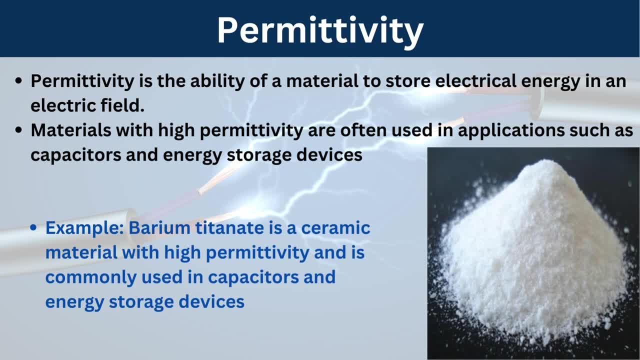 electrical energy in a electric field. okay, so the material with the high permittivity are often used in the application, such as capacitor and the energy storage devices. okay, so barium titanate is the ceramic material with high permittivity and are commonly used in the capacitor and the energy storage. 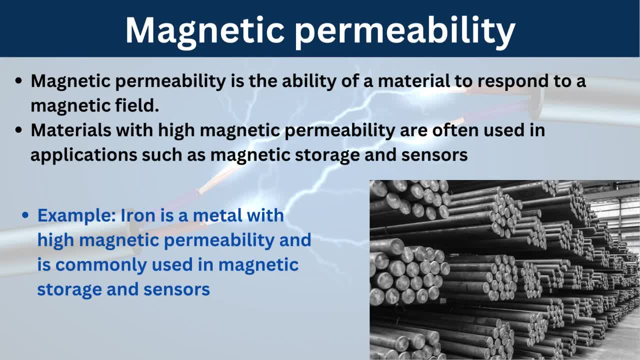 devices. next, electric property is the magnetic permeability. okay, so the magnetic permeability is the ability of material to respond to a magnetic field. okay, so the magnetic permeability is the ability of material to respond to the magnetic field. okay, so the material meter high magnetic permeability are: 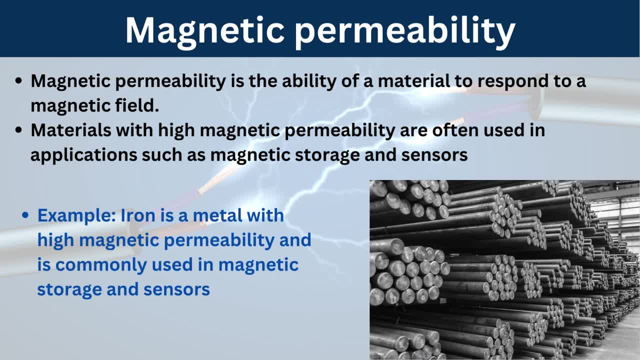 often used in the application, such as magnetic, stronger magnetic energy and see. on the other hand, these are the kinds of ользa makeskill-ipAlright- I will mention it in a plenty of time- in the storage and the sensors. okay, so you can take the example here. the iron is the metal with 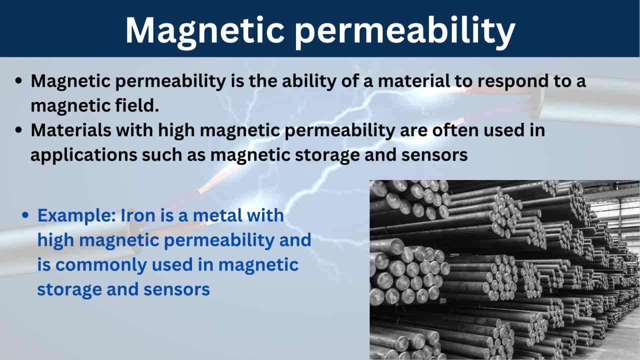 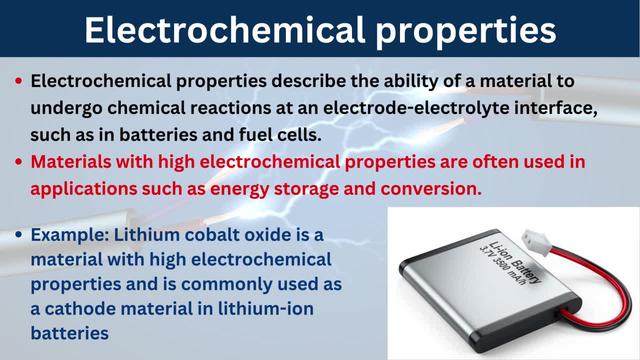 the high magnetic permeability and are commonly used in the magnetic storage and the sensor. next property is electrochemical properties. okay, so the electrochemical properties describe the ability of material to undergoes chemical reaction at an electrode electrolyte interface, such as in battery and in the fuel cell. okay, so the material with high electrochemical 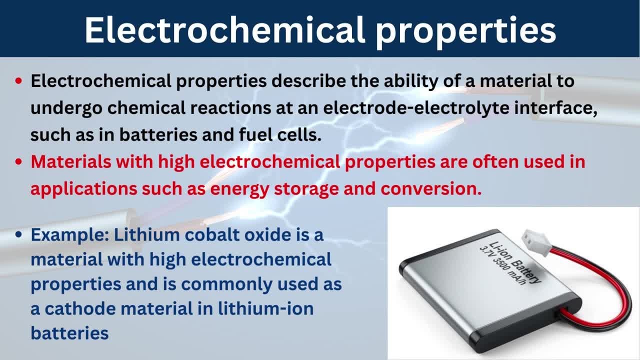 properties are used in the application, such as energy storage and the convergence. so the lithium cobalt oxide is the material with the high electrochemical properties and it is commonly used as a cathode material in the lithium batteries. so the lithium cobalt oxide is the material with high electrochemical properties and it is commonly used as a cathode. 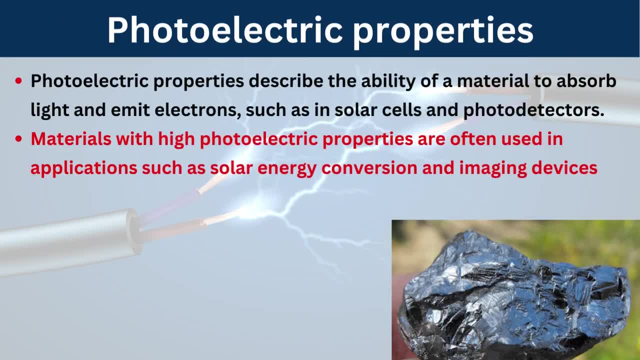 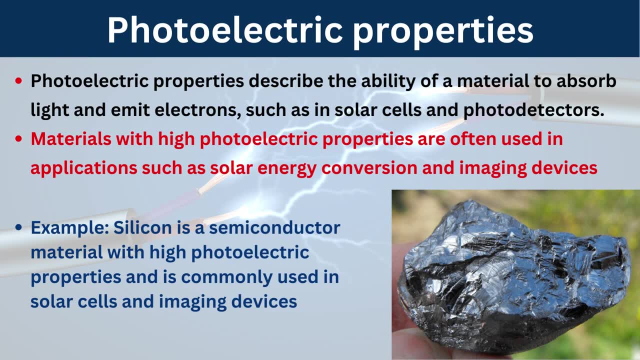 material in a lithium ion batteries. next electrical property is the photoelectric properties. so the photoelectric properties describe the ability of material to absorb light and emit the electrons, such as in a solar cell and the photo detectors. okay, so the material with properties are used in the application, such as solar energy convergence and and.